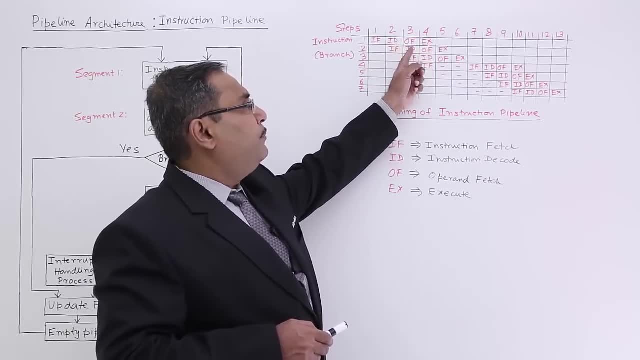 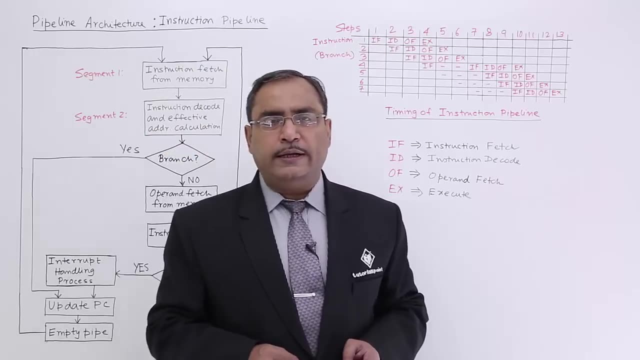 will go to the operand fetch. second instruction will come to the instruction decode and third instruction will be coming for the instruction fetch. Obviously, we know that in case of pipeline architecture, instructions are getting executed phase wise, interleaved. Now, that is a certain 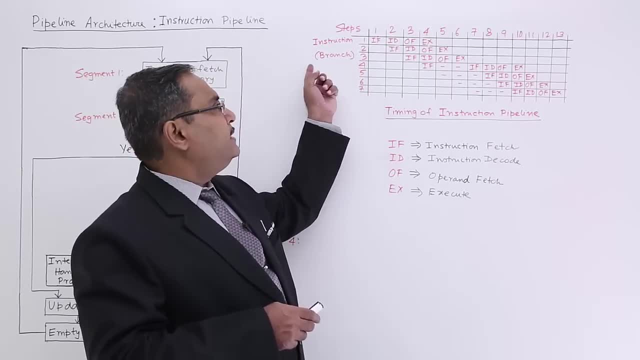 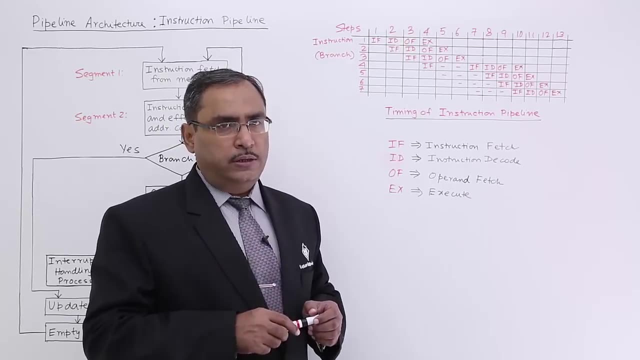 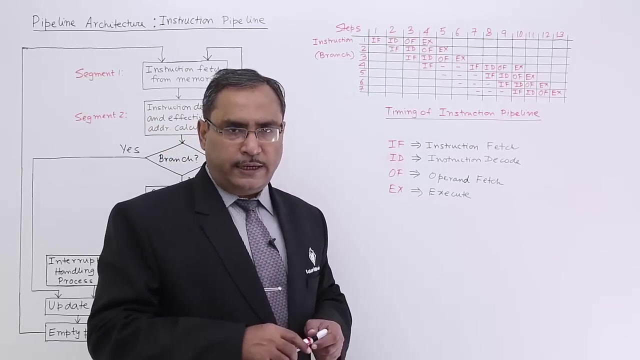 condition, Say on the third instruction. this instruction is category. is having the category ganch or jump instruction conditional or unconditional? ok, Then what will happen? The linear or the sequential execution of instructions will get hampered for that. As a result of that, the next instruction, which is just after the third instruction, 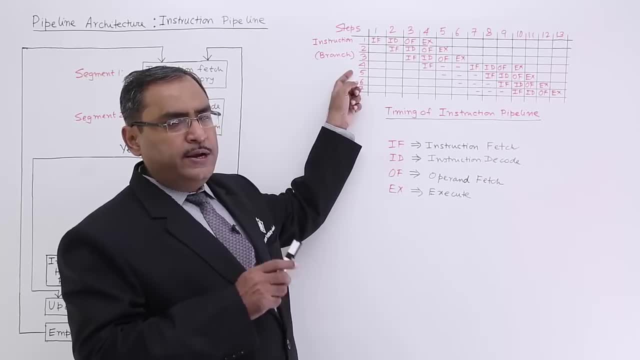 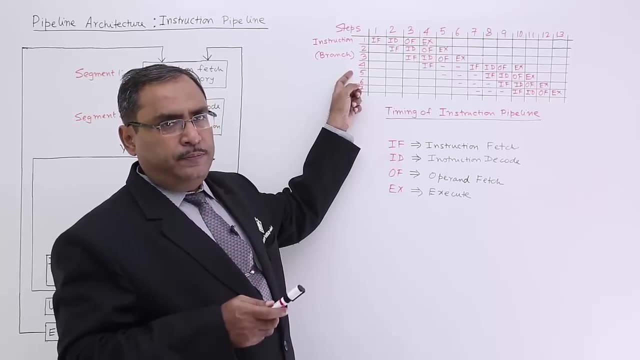 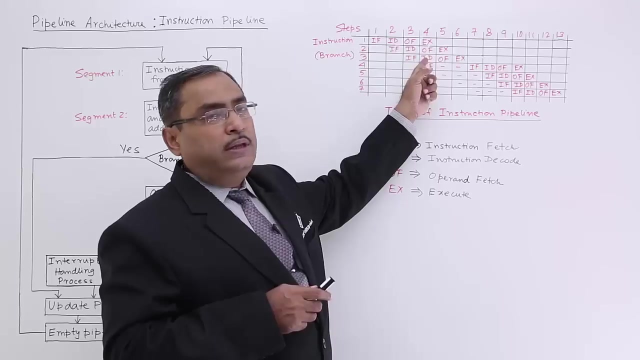 in the program will not get executed because, due to the presence of the jump or go to instruction, the program control is supposed to get transferred to a different memory space, target memory location. But that will remain unknown until I decode the branch instruction. So the next. 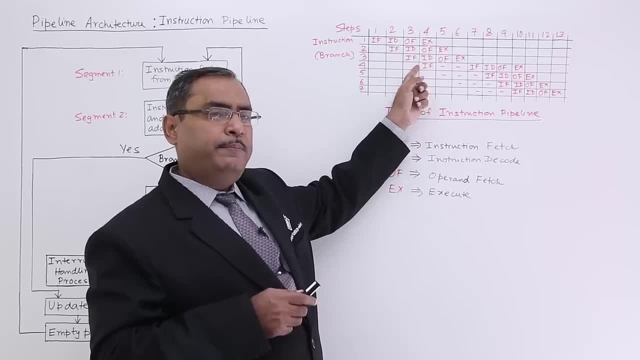 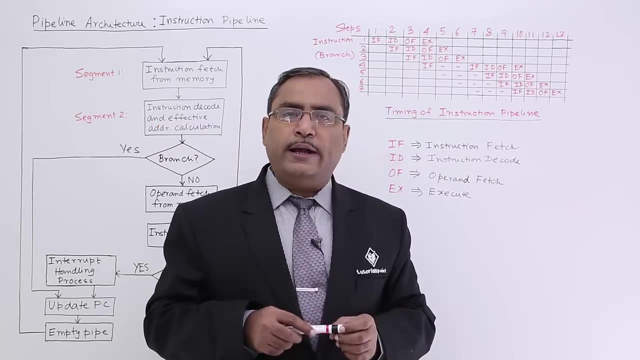 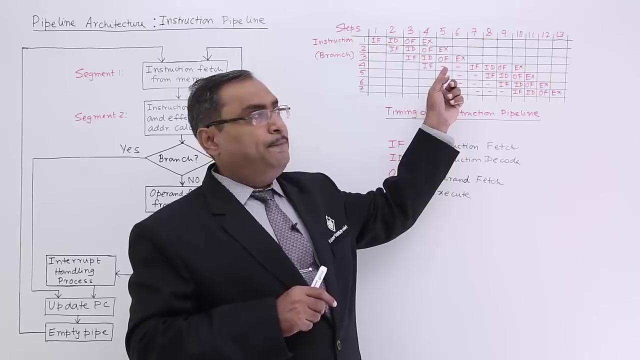 instruction from the program will be fetched in the minimum. But after decoding the processor will be able to understand that next instruction is not going to get its control. So as a result of that, this instruction execution will be blocked and these phases, these particular cycles, will remain unutilized. for the fourth, 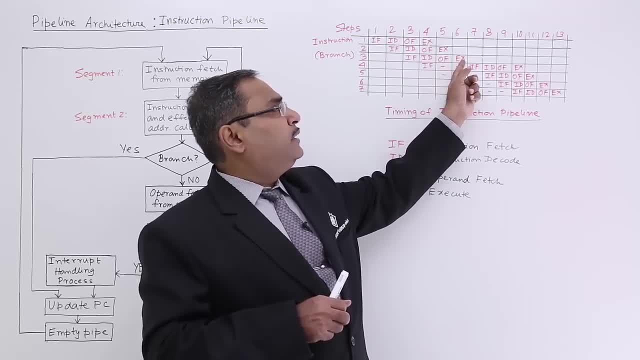 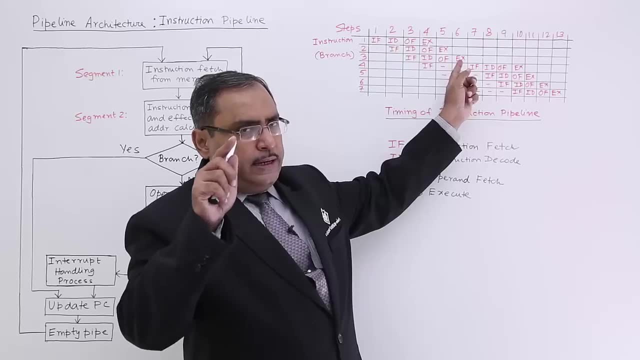 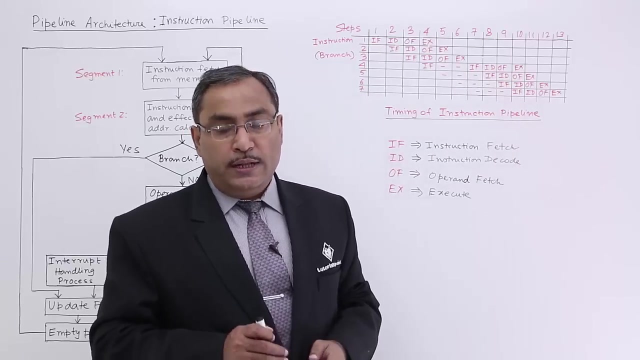 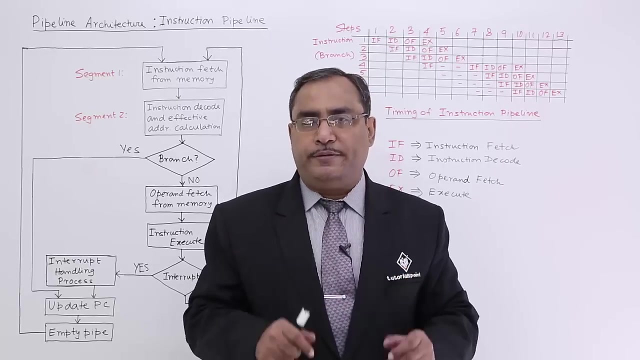 instruction. So after completion of the third instruction, when it will be sure that instruction control is going to that particular target address, Then from the target address the next instruction will be fetched and the process will be resumed. This is known as pipeline stall, So pipeline has got halted. So as a result of that, you 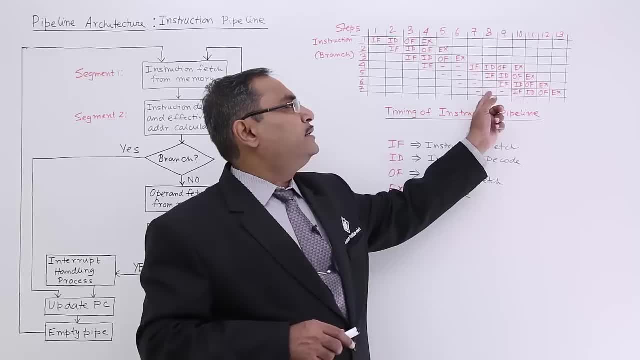 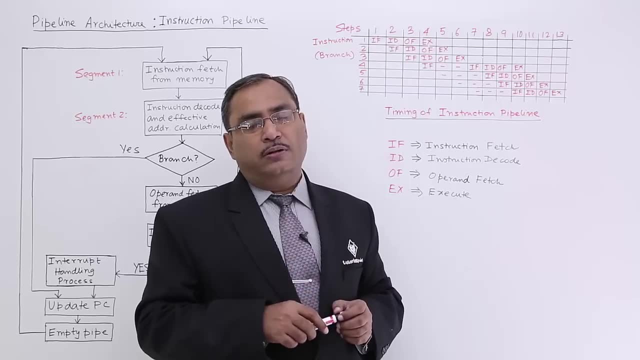 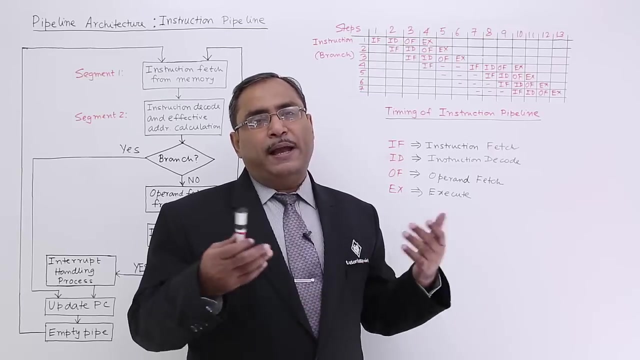 see, so many phases are there, so many time cycles were there for which this pipeline remain unutilized, and this is known as pipeline stall- And obviously that when the pipeline stall will take place, the pipeline efficiency will get decreased, The pipeline throughput will get decreased and that will be the deterioration. 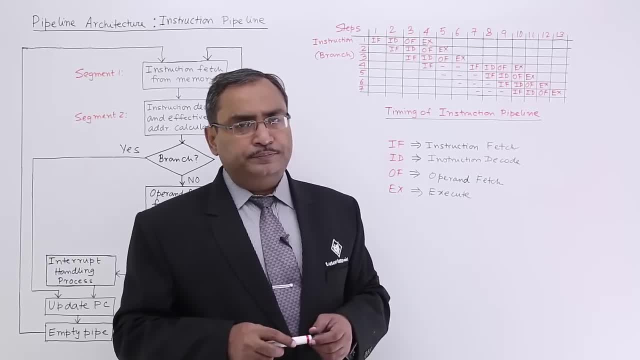 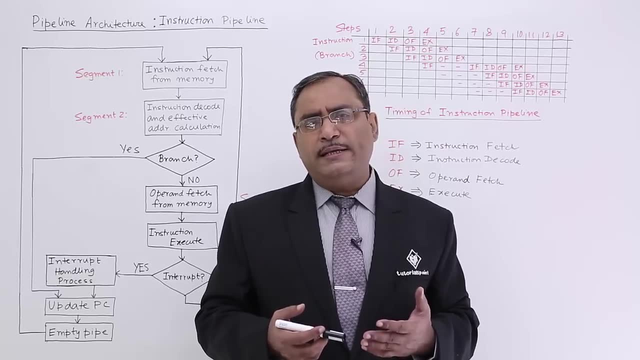 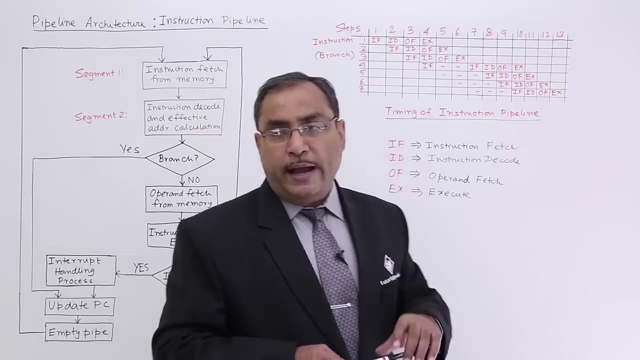 in the performance of the pipeline. So obviously, due to the introduction of so many branch andども resulting instructions in pipeline architecture, the program execution performances, performance parameters, will get degraded. So I have discussed this particular timing diagram. Now come to this particular 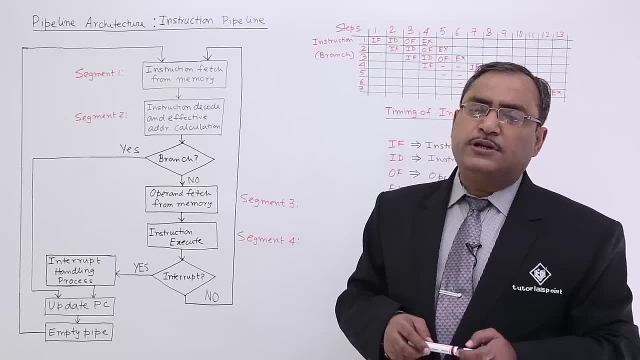 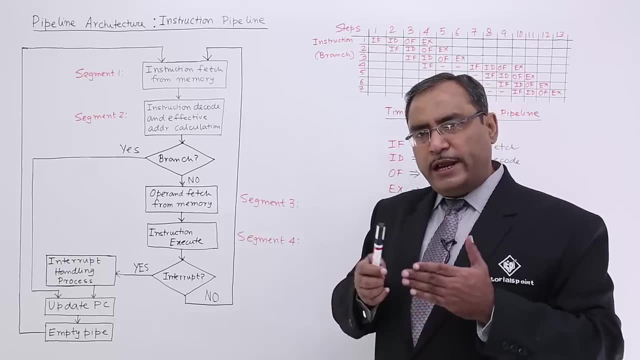 flowchart. So in the segment one, what will happen? The instruction will be read. from where? From the memory. In the segment number two, what will happen? The instruction which has been read. the instruction which has been read will be decoded. 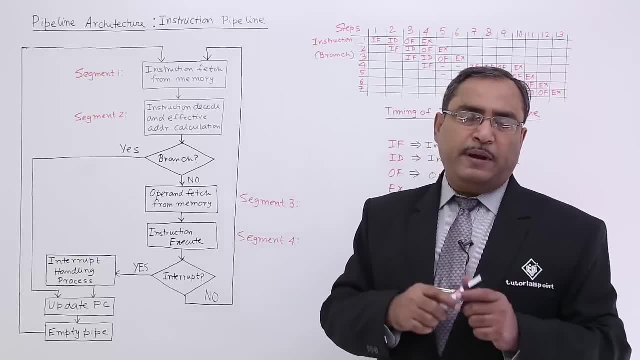 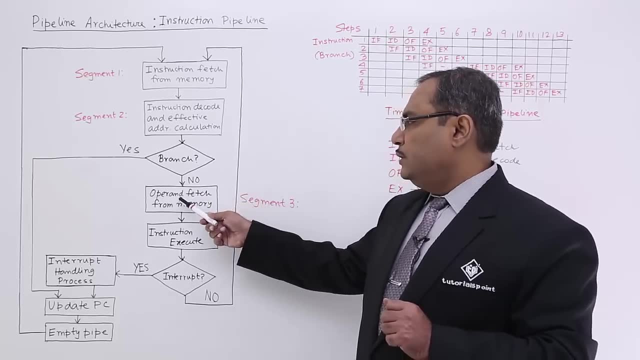 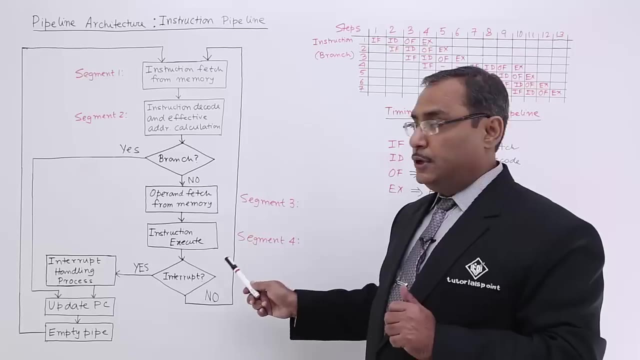 to get the meaning of the instruction And it will calculate the effective address of the operand. Is it a branch instruction, Say, for the first time, I'm considering no, Then the operand will be phased and instruction execution will take place. So four segments have got completed. 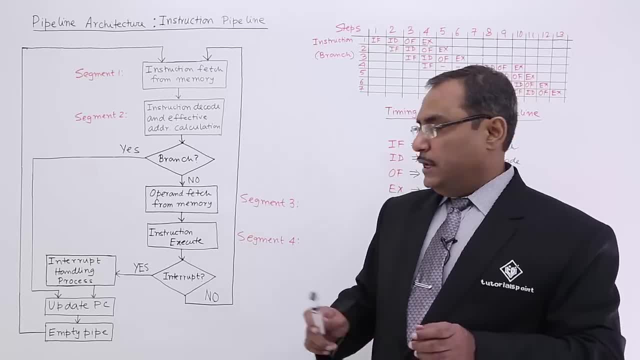 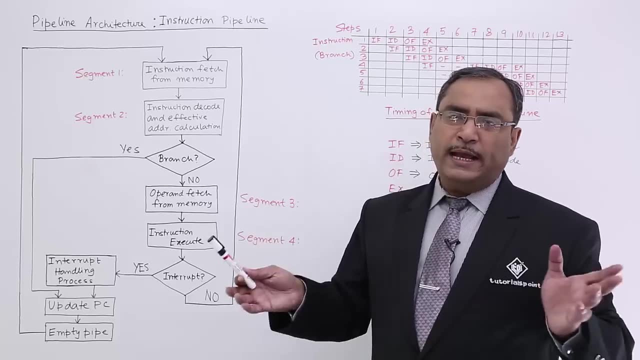 Now it will check whether any interrupt is pending or not. If there is one interrupt, then it will be processed. Otherwise, the next instruction will be phased and will be executed accordingly. But if it is a branch instruction, then pipeline stall is going to take place. 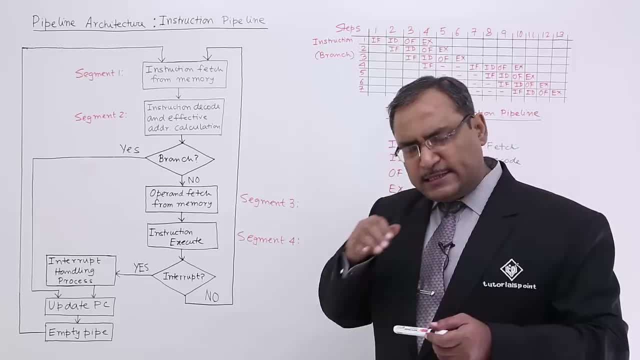 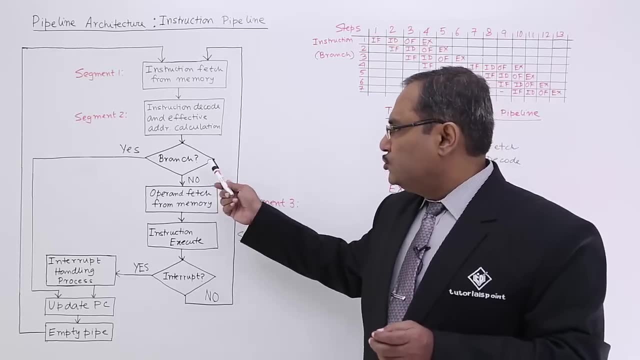 What is the meaning of the term pipeline stall? Pipeline stall means the next instruction, execution will be cleaned up, The pipeline will be made empty, And that is known as a pipeline stall. So, yes, if it is yes, then update the program counter. 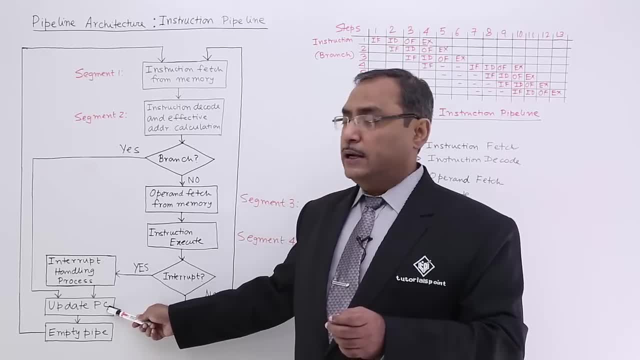 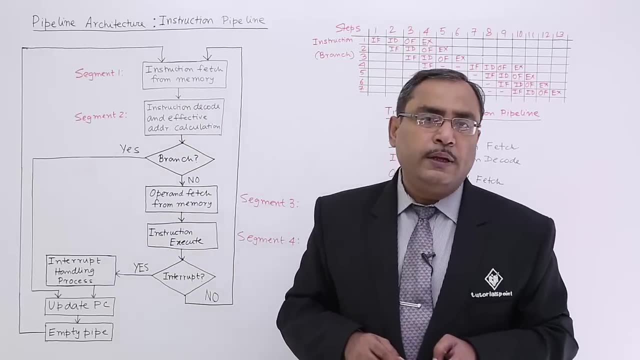 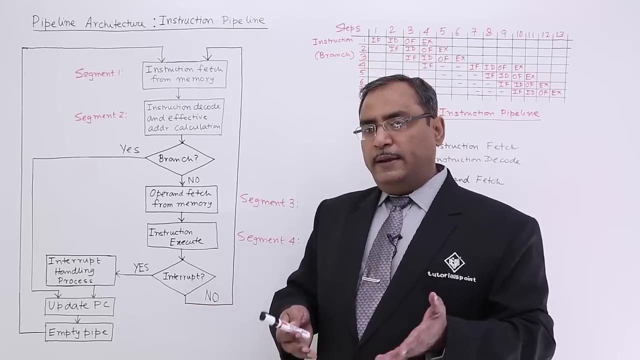 with the target address, from where the next target instruction has to be read and executed, And then empty pipe will take place And then the process will be restarted And if interrupt has occurred, then also the program is now getting postponed or suspended. The program control will be going to where? 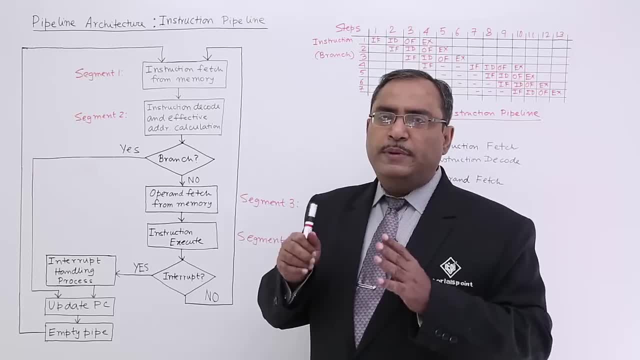 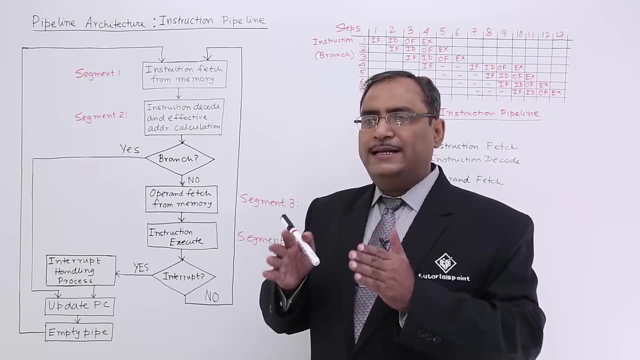 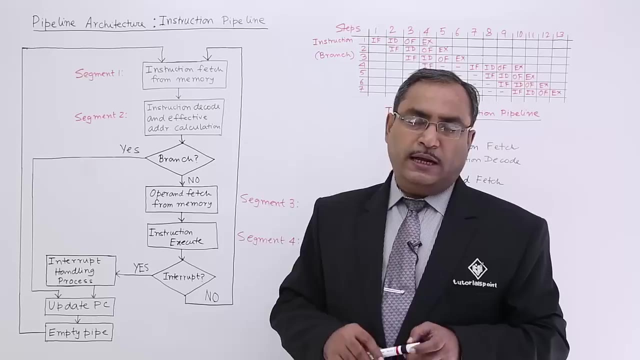 To the interrupt handling routine. So the routine means the procedure, the program, the program segment which is supposed to get executed to handle the interrupt for what it has been caused. And so again, the empty pipe will take place after updating the program counter. 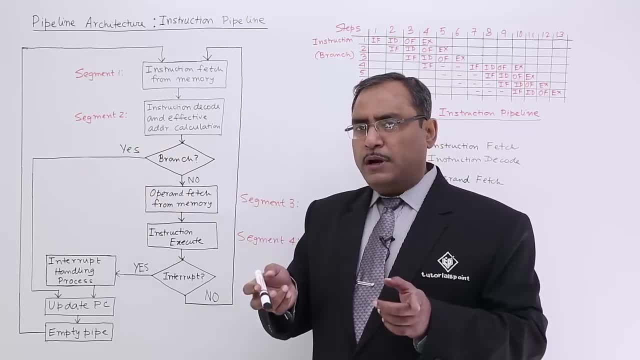 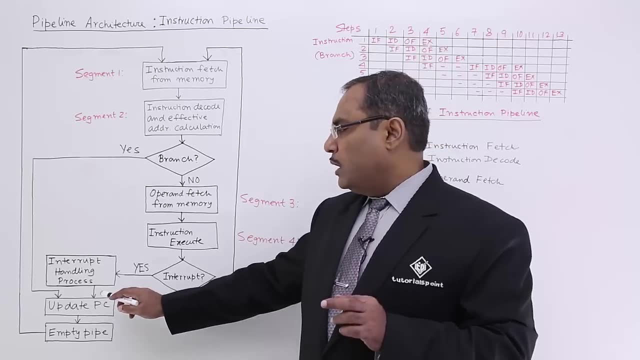 That means please go to that particular address. We know the program counter is nothing but a register which will hold the address of the next instruction getting executed. So the program counter has to be updated with the starting address of the interrupt handling routine or it will go to the interrupt table. 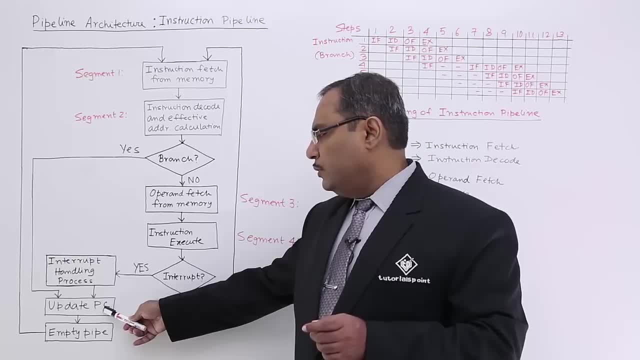 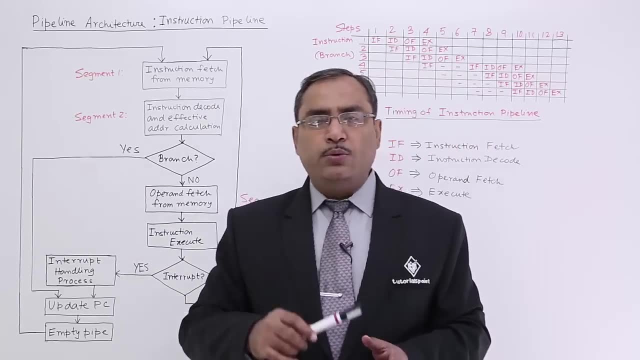 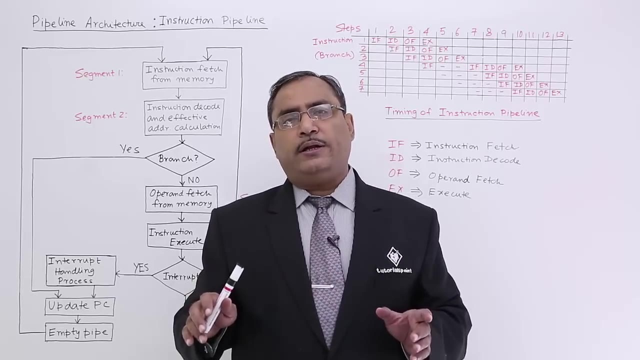 So now this update program counter will take place And then empty pipe again. the pipeline stall is going to happen And the process will be restarted again with the new target address, new target instruction from the address. So in this way the instruction pipeline will get executed.